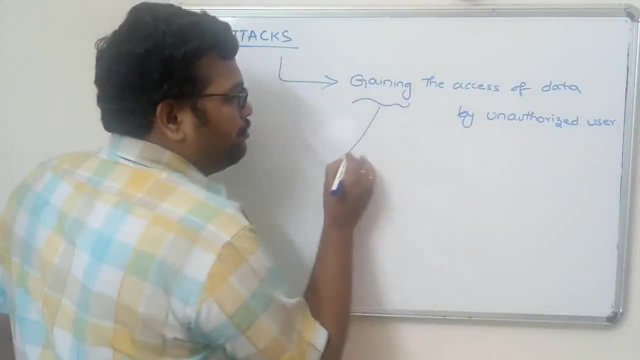 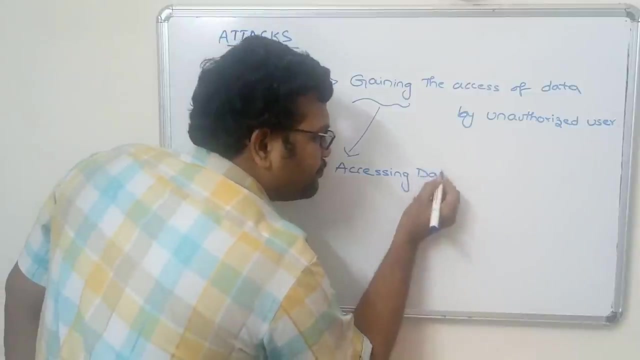 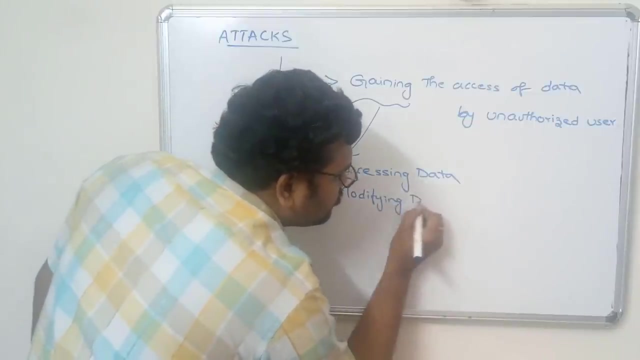 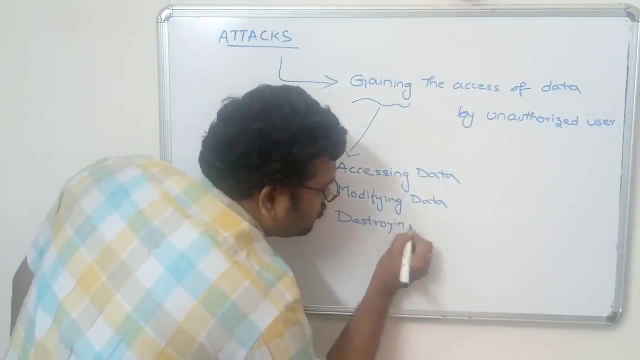 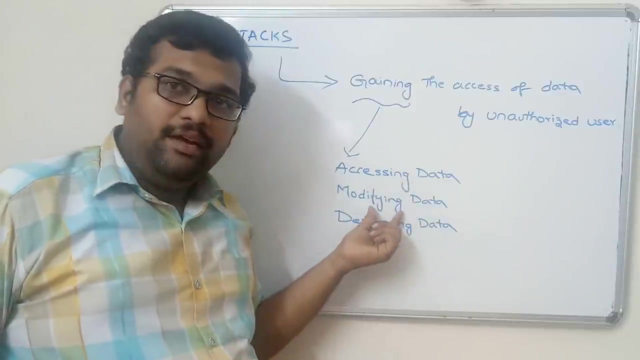 call it as attack. Here the word gaining the access of data by unauthorized user is means accessing the data, modifying the data, destroying the data. So, whatever it may be accessing or modifying or destroying the data, whatever it may be accessing or modifying, 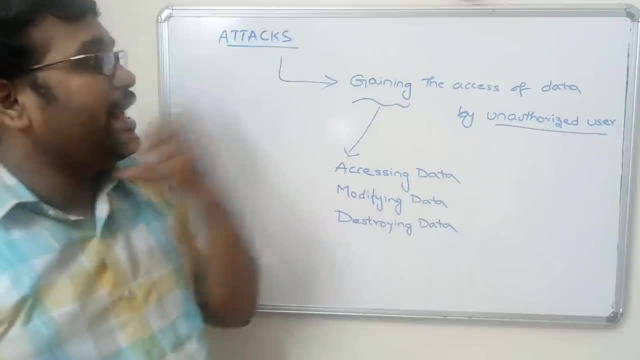 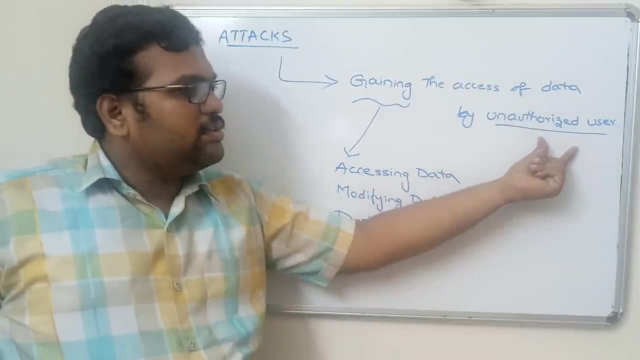 or destroying the data means. So these are several different ways ofięing data. in network, the data is co-defining and attack is gaining the access of data by unauthorized user, so this unauthorized user may directly access the data or modify data or destroy the data here there. 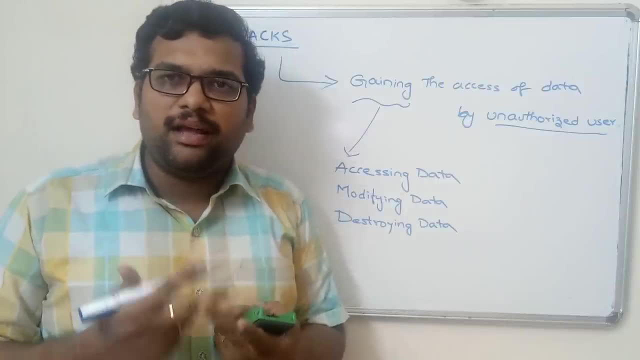 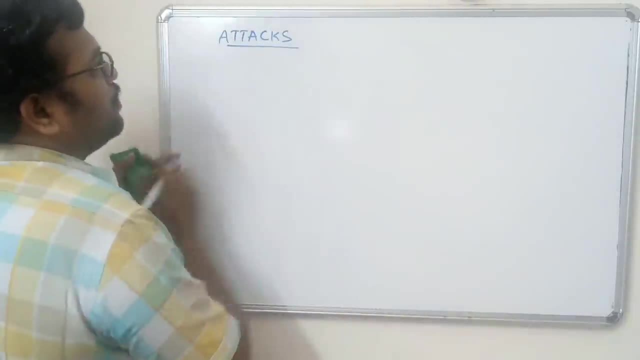 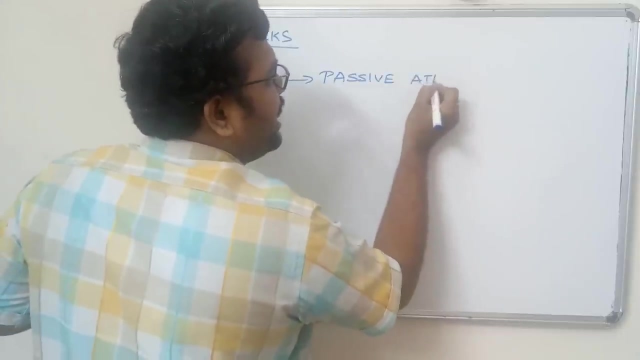 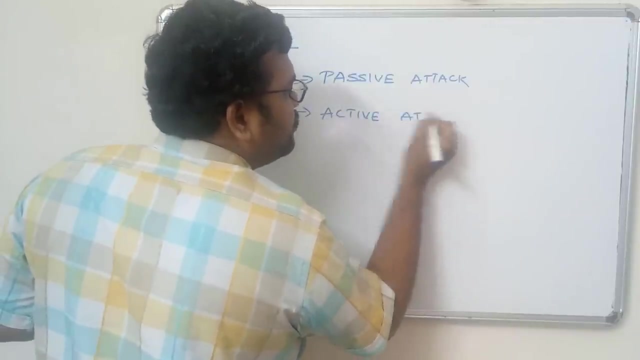 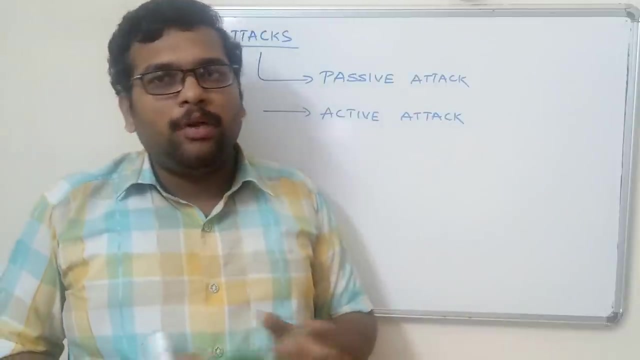 are two categories of attacks. one is passive attack, another one is active attack. these are of two types. one is passive attack and active attack. so here the passive attack means the data will not be modified, just the data will be accessed by the third person, the third person. 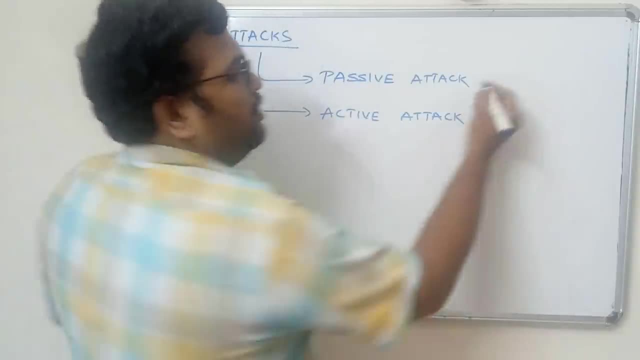 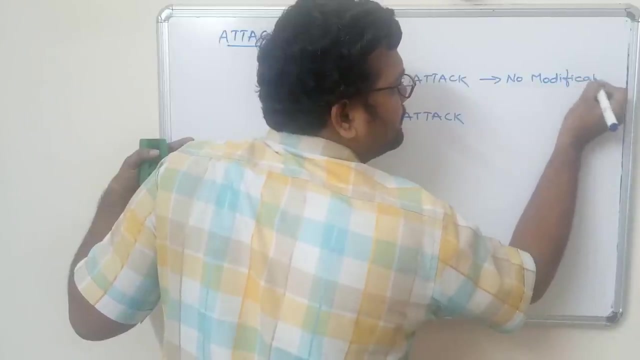 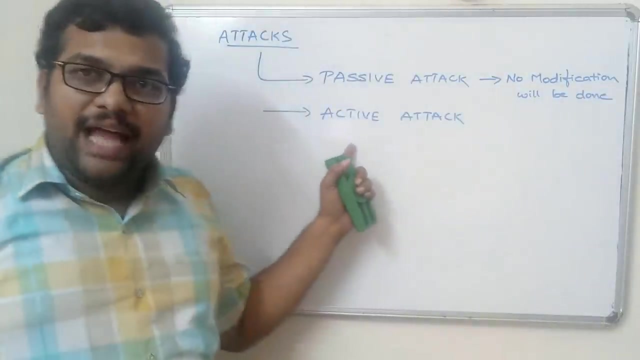 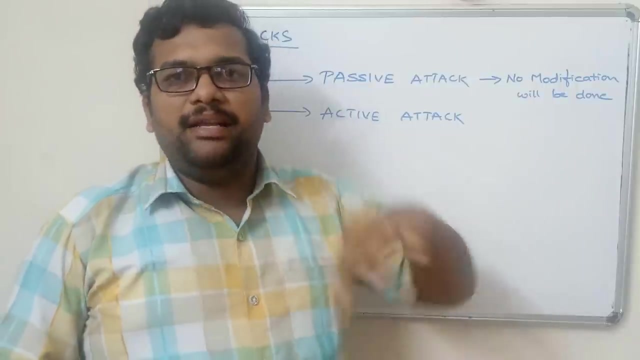 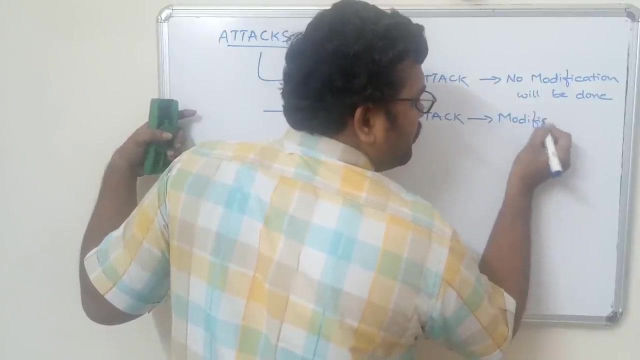 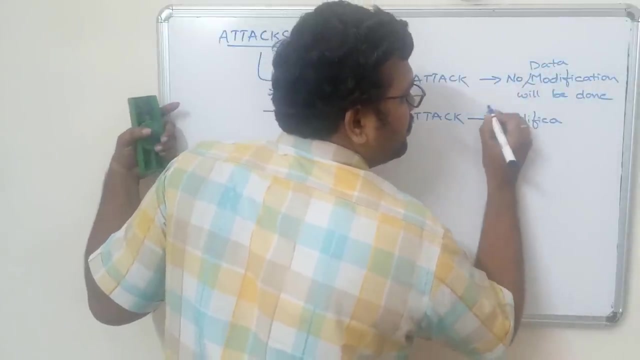 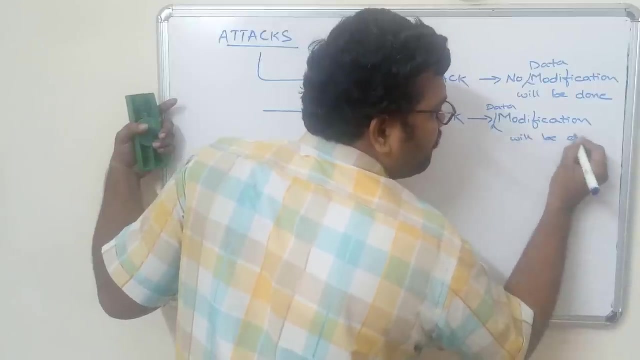 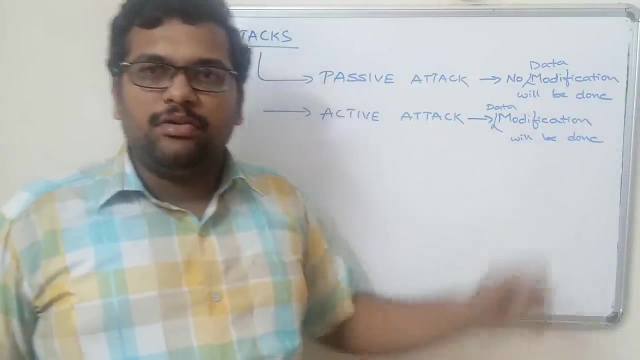 is unauthorized person. so here no modification will be done. and coming to this active attack, the name itself indicates it is an active attack. that means here the data will be modified by the unauthorized user, so here modification will be done. data modification, so no data modification will be done. and here the data modification will be done. so the final: 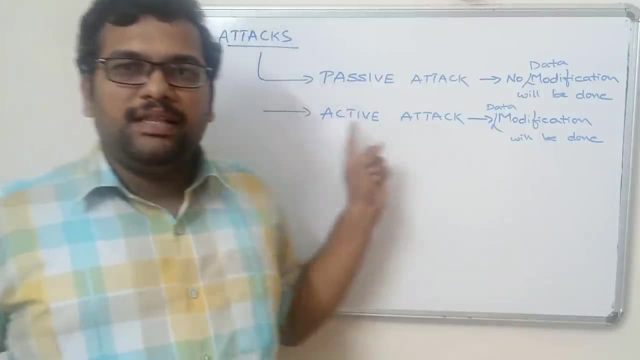 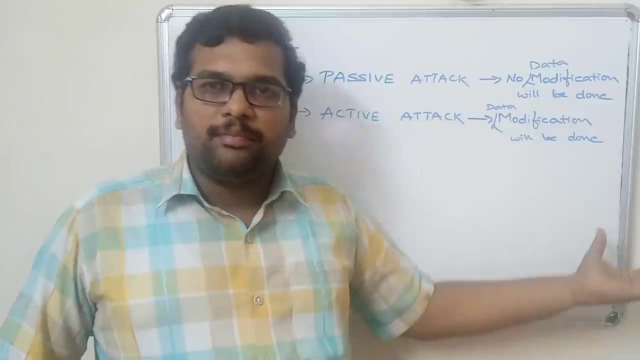 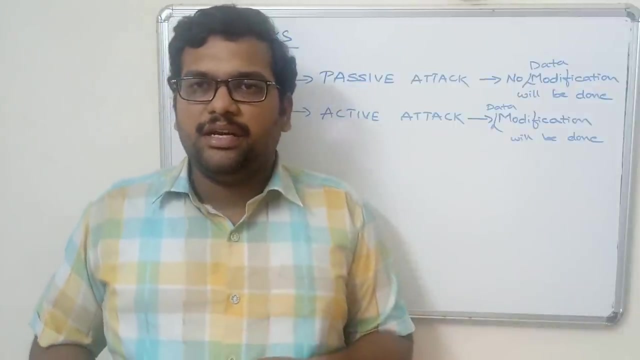 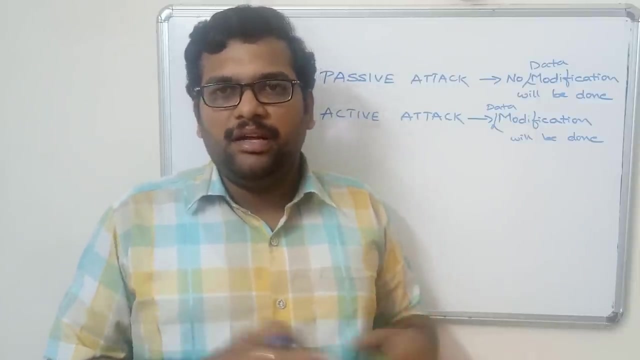 impact will be more for this. active attacks because the data will be modified and that modified data will be received by the user. so if sender sends the message and receiver receives the message, the sender sends one message and the receiver receives another message which is modified by the unauthorized user. those attacks, we call it as active attacks and passive attacks. 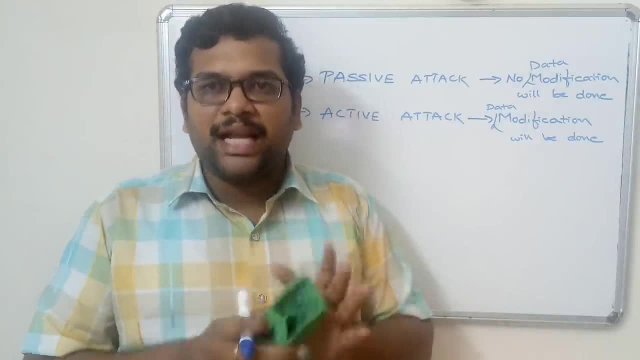 are no data modification will be done just they will access the data coming to this activate path whenever the��게 approach is qualidade additional result is only if the reconciliation between number of layers of data is과 in response the mới track of respect this will be longer the second factor the � tasked warning your 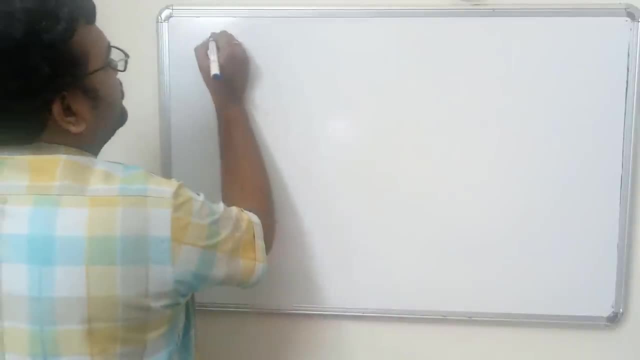 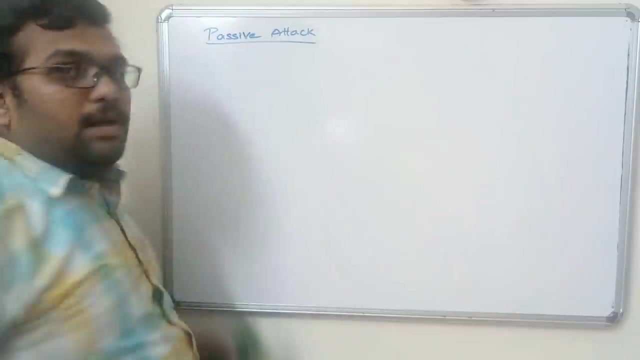 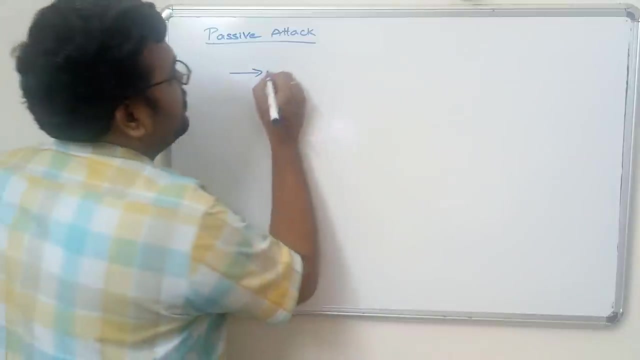 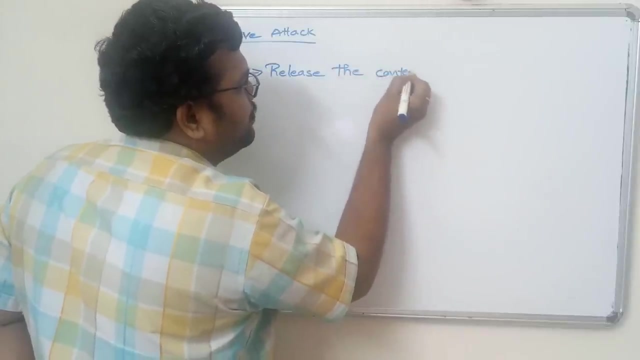 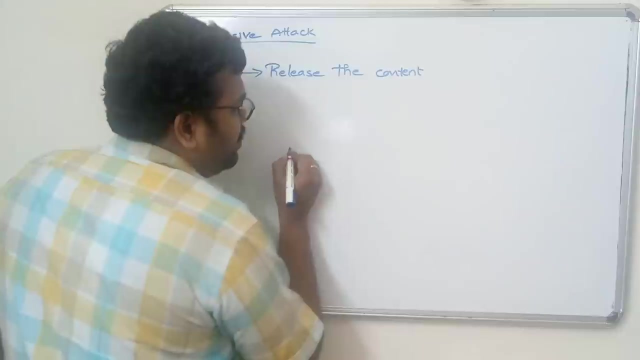 so that modified data will be received by the user. so if sender sends the message and the receiver receives the Coming to this passive attack, there are two methods for this passive attack, two techniques. One is release the content. releasing the content, that means this is the sender and 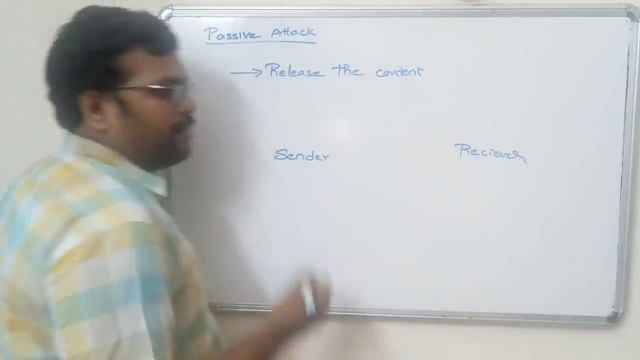 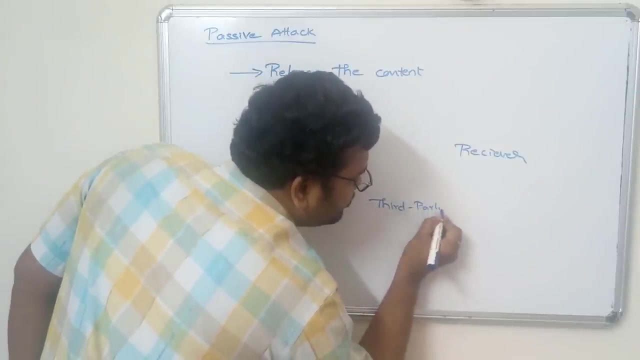 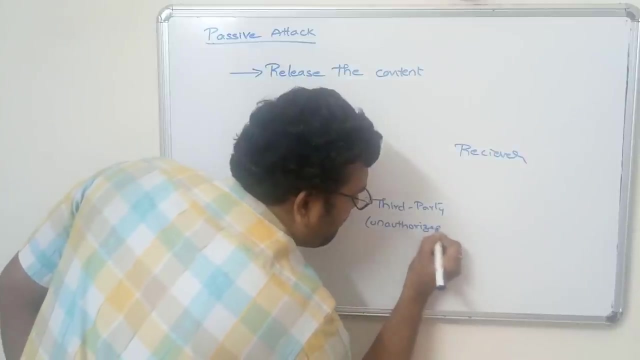 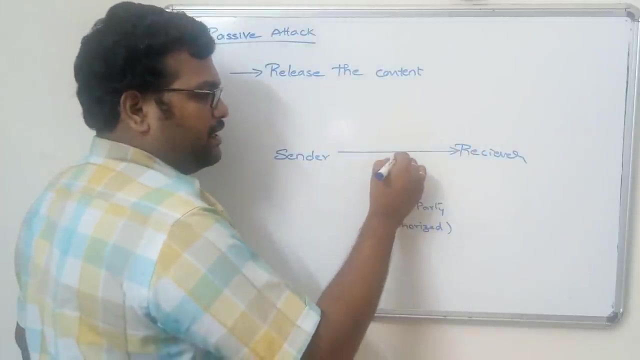 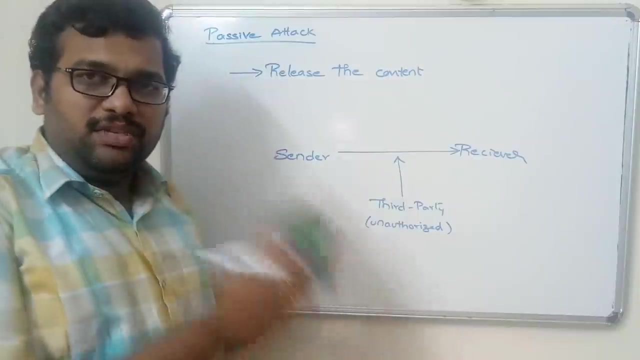 this is the receiver, This is the third party. This is the unauthorized access. this is the unauthorized access. So if the data is sent to the receiver, the third party will just access the data. That means by listening or using some other techniques. he will gain, he or she will gain. 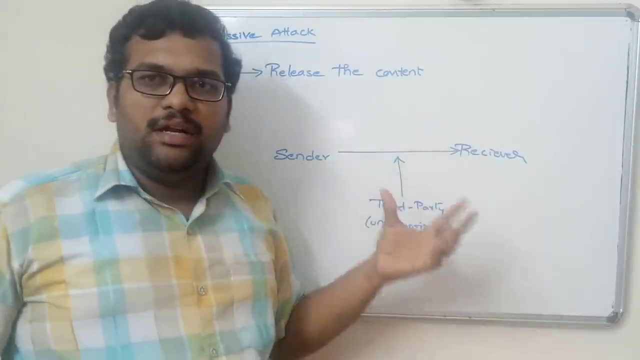 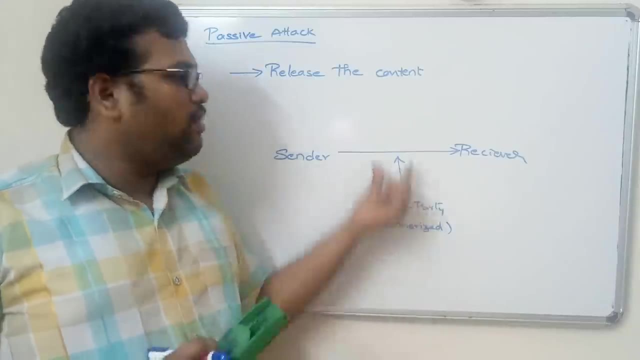 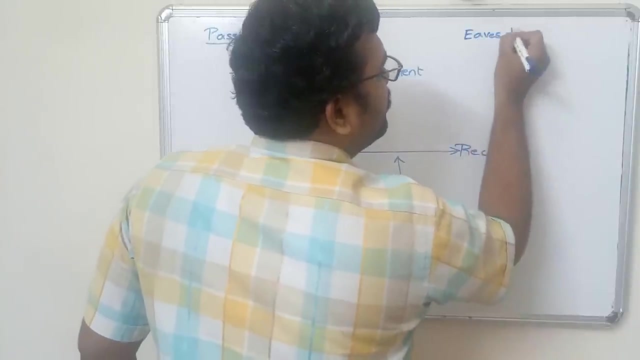 the data which is sent by the sender to the receiver. So here there will be no modification, Just this third party will get an access of this data. These type of techniques we call it as eavesdropping. eavesdropping technique. that means no modification. 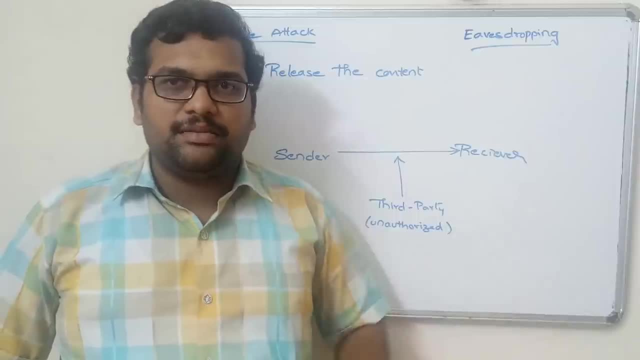 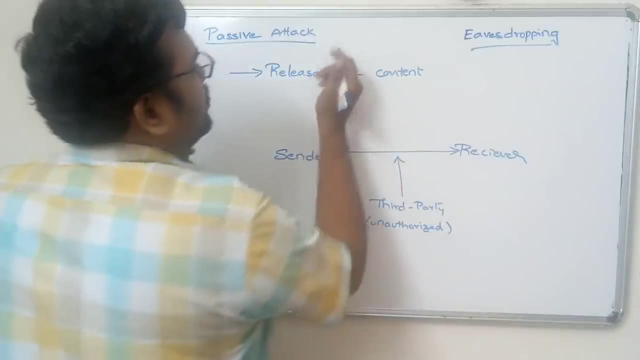 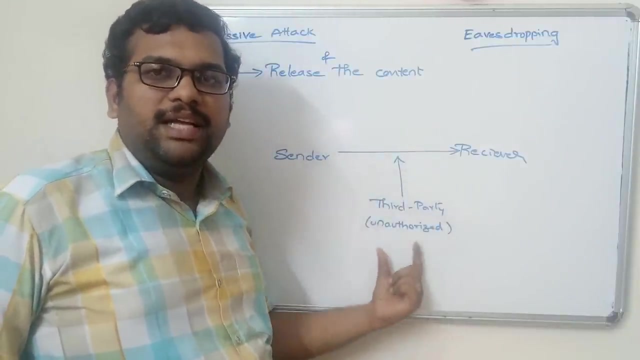 will be done. Just they will listen to the messages. So this is the release of content: release of the content. So this is the release of content. So this is the release of content. So this is the release of content. So the content will be released. that means accessed by the third party that is unauthorized. 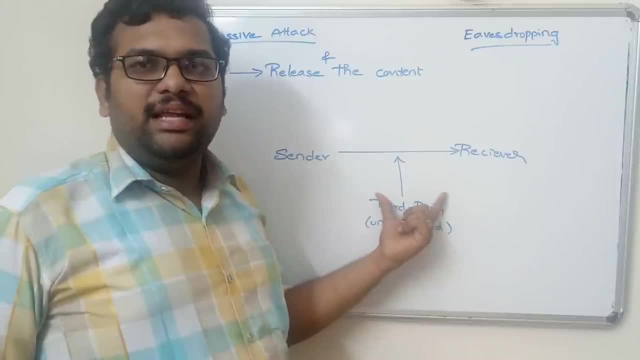 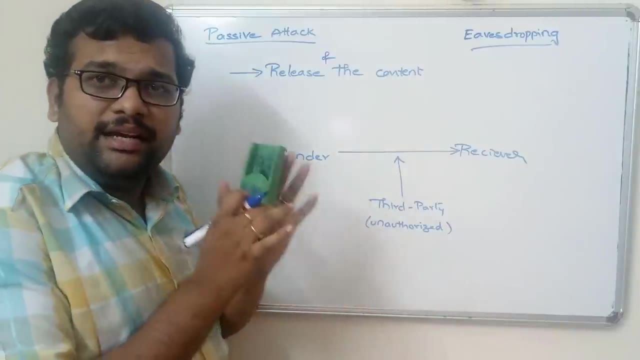 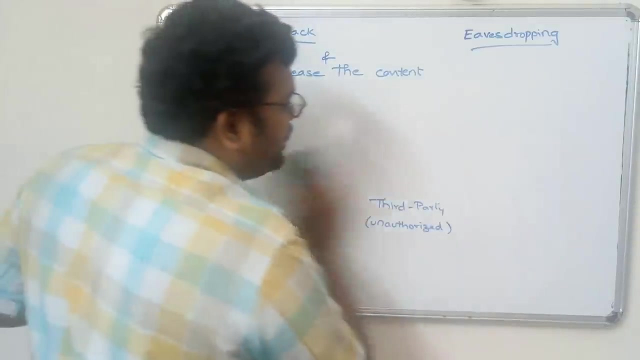 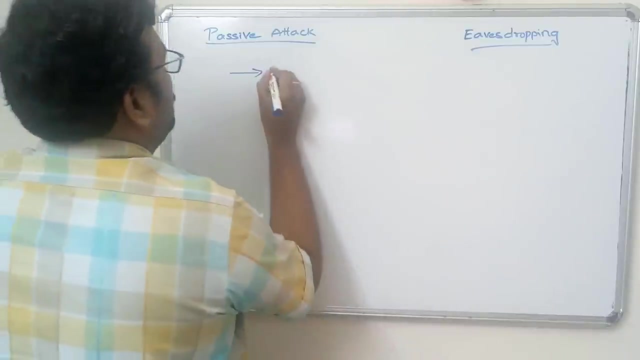 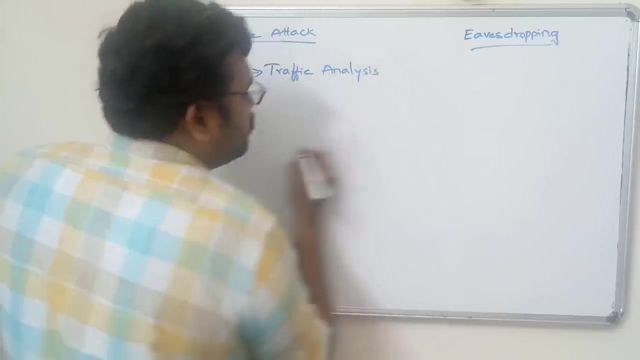 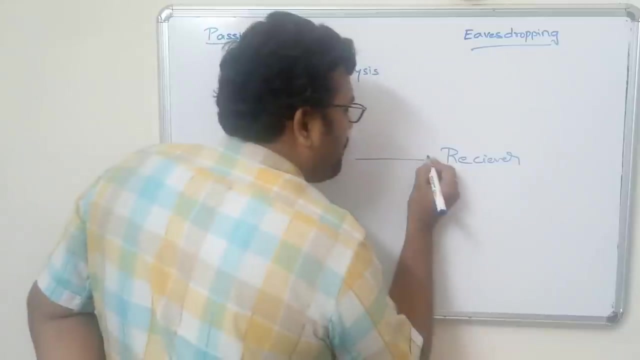 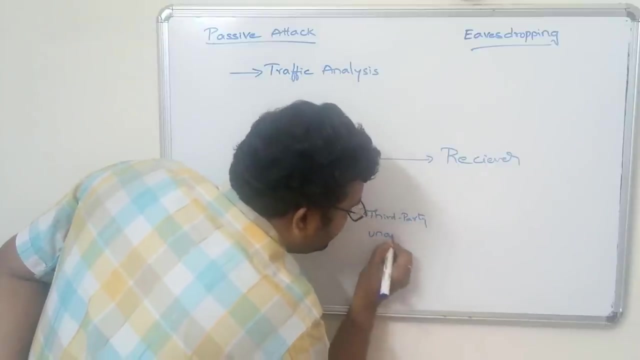 access. So there will be no modification, just it is a eavesdropping technique, Just the third party will observe the messages and he or she will gain the access. that's it Coming to the second category, Traffic analysis. So here also the sender will send the message to the receiver and third party. that means 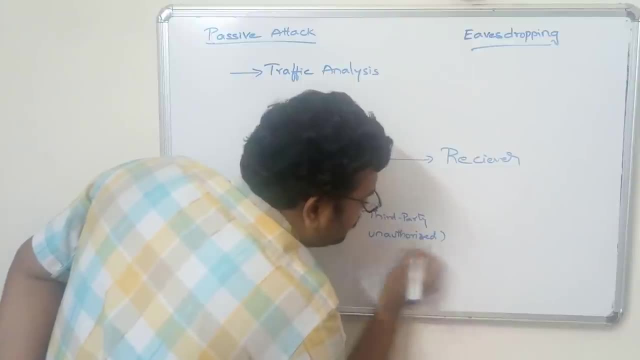 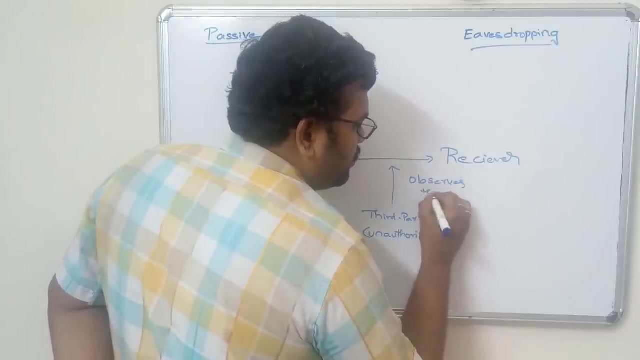 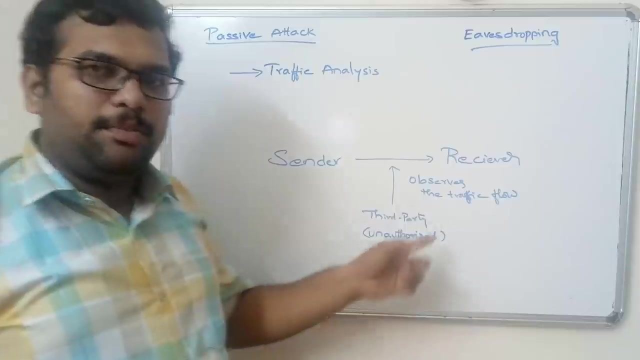 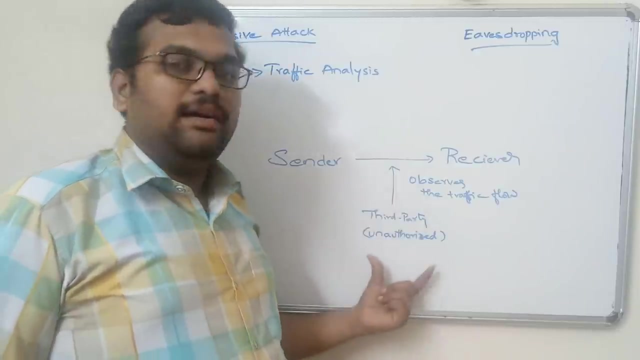 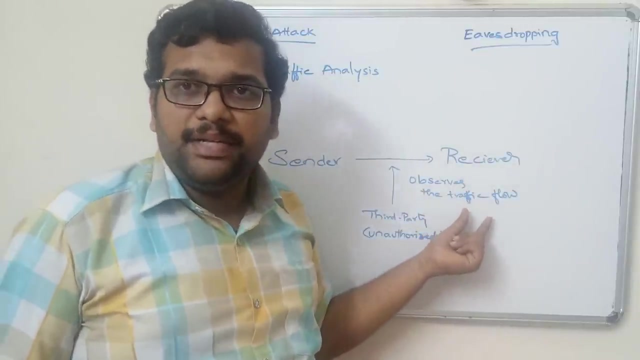 unauthorized access. unauthorized user. Just authorize the user. Just authorize the user. Just authorize the user. Observes the traffic flow, Traffic flow and, based upon this observation and based upon this traffic, third party or unauthorized person will access the data. So, based upon the traffic between the sender and receiver- here the traffic, the word traffic- 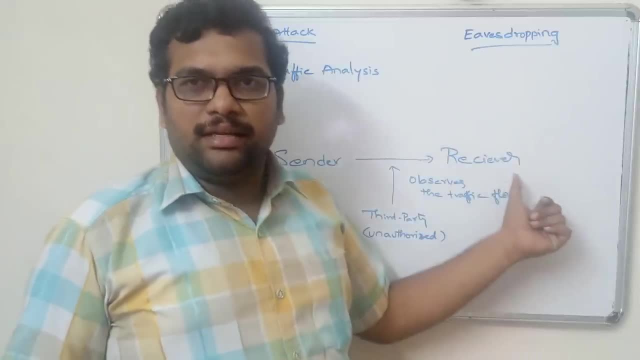 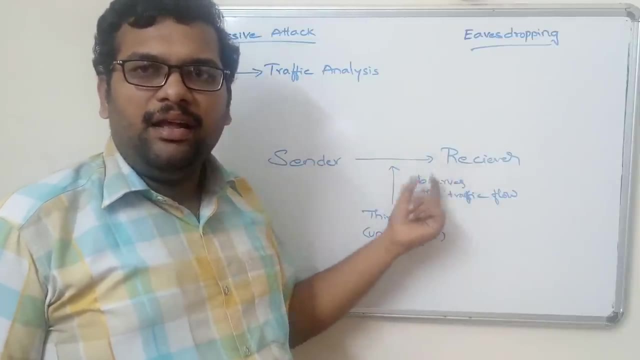 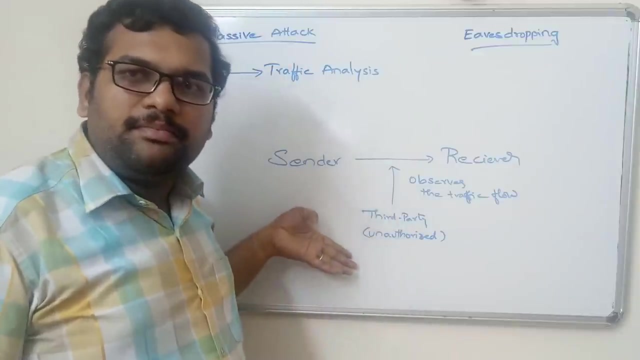 means data sent by the sender to the receiver. So based upon the traffic between the sender and the receiver- here the traffic the word to the receiver. so keep on monitoring the traffic between center and receiver and the another person will access the data. so he in this process also there. 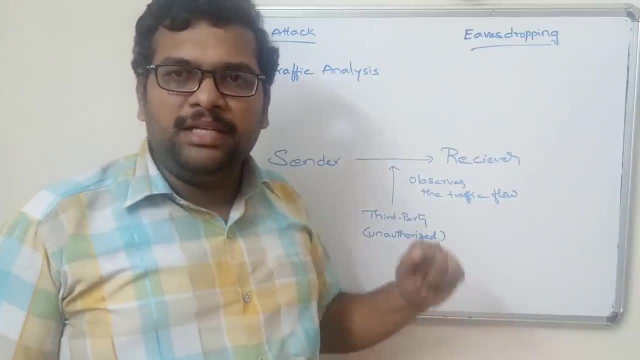 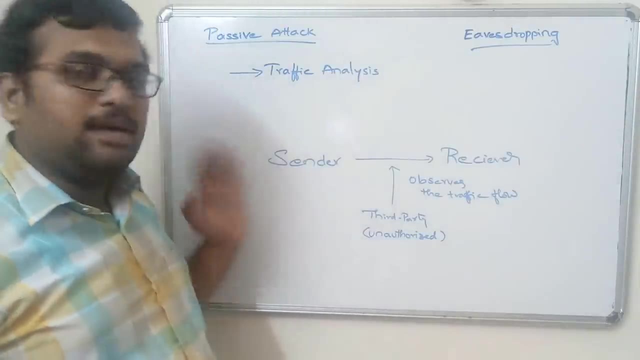 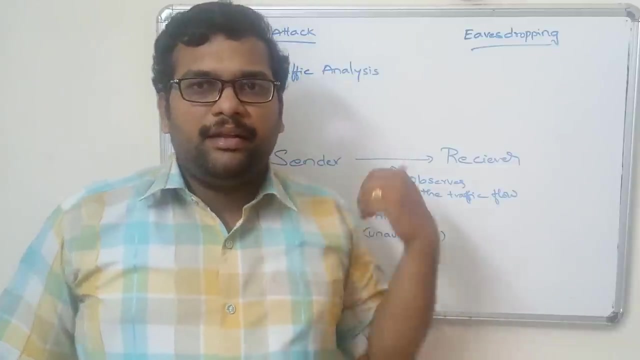 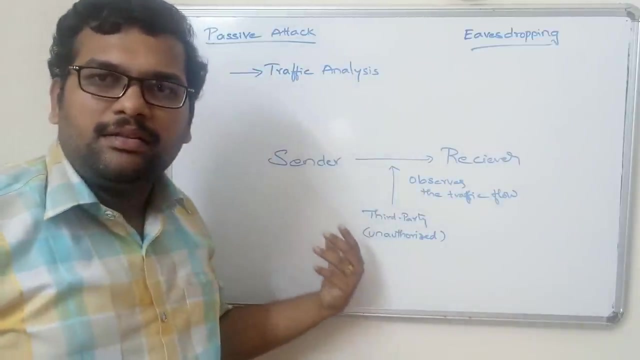 will be. no modification will be done on data. so that means it is also one type of eavesdropping technique. so these two comes under passive attacks. one is release, releasing of the content, and the second one is traffic analysis. in the releasing of the content, just the content will be accessed by the third. 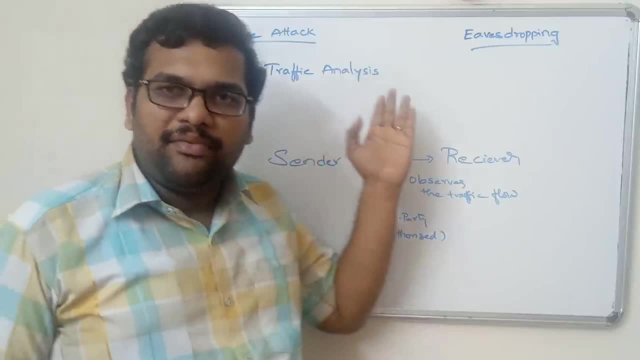 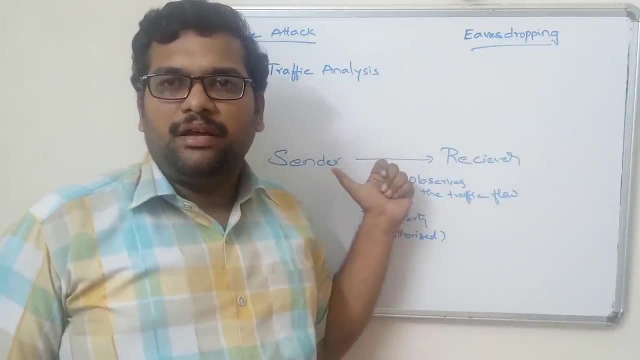 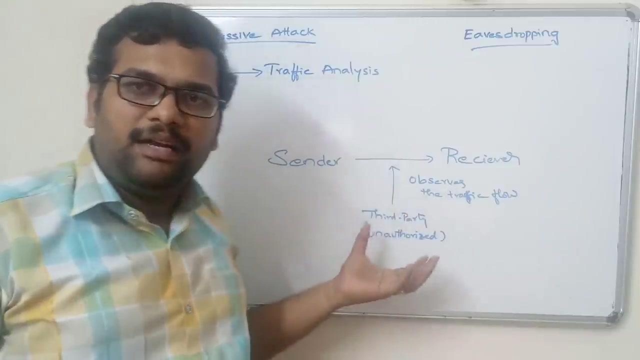 party. so no modifications will be done. and here the traffic analysis. the third party will keeps on monitoring the traffic in between the sender and receiver and based upon the traffic flow, the third party will gain the access. that will see, the third party will get the data. so here also, no modifications will be done. so that is. 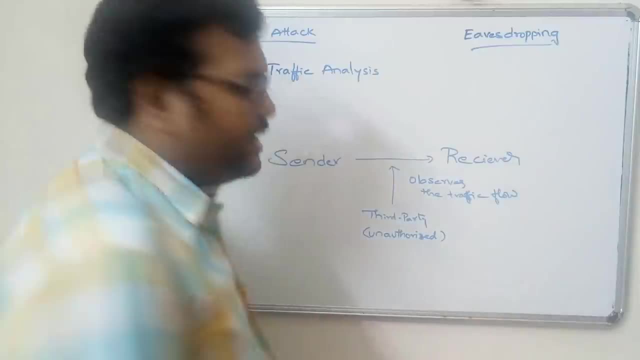 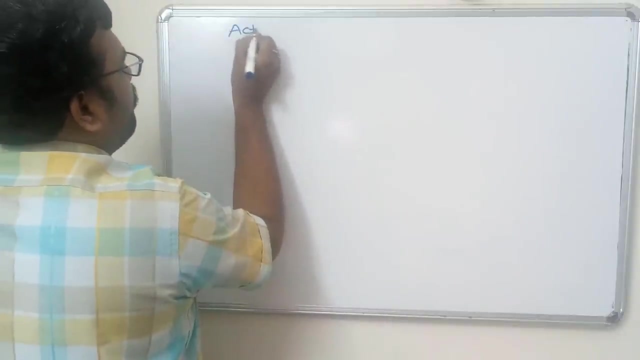 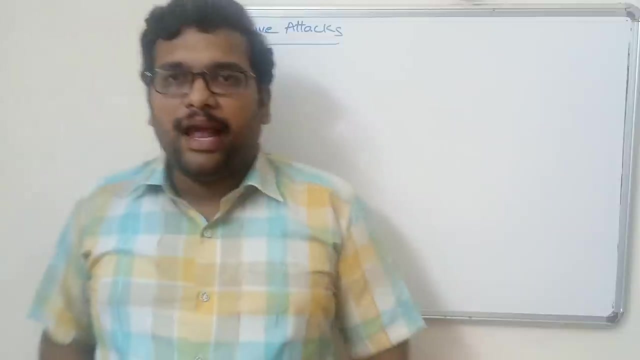 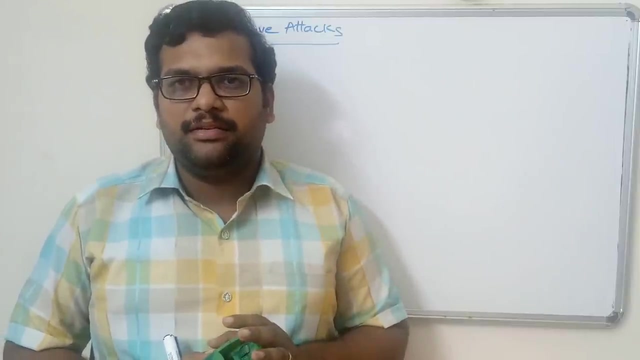 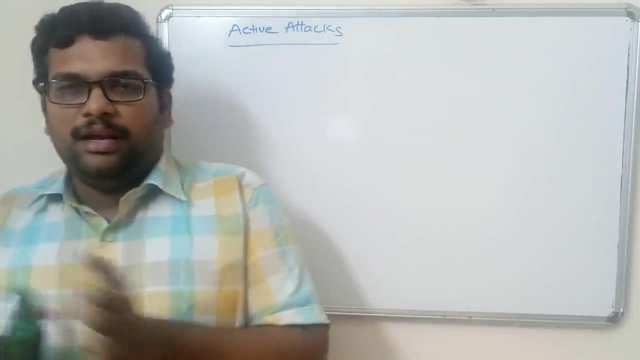 passive attacks. coming to the next category, that is, active attacks. so here, active attacks, the modification will be done on the data by the unauthorized person. so if sender and receiver are the authorized persons, if sender sends the data from the, I mean if the sender sends the data to the receiver. so in between, 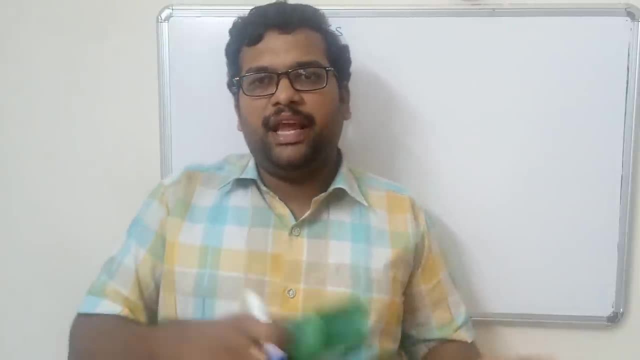 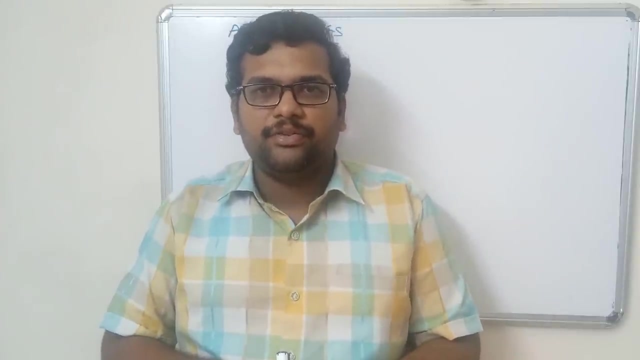 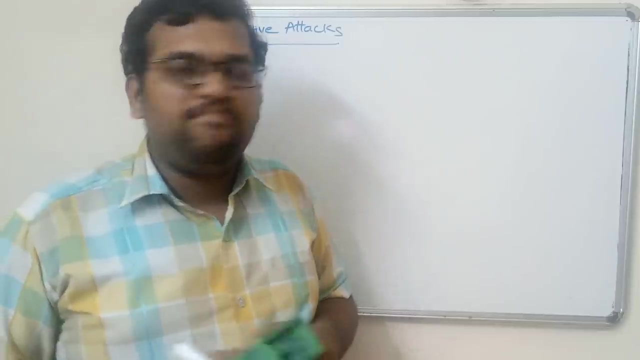 the transmission, the unauthorized person will gain the access and the person will modify the data in between the transmission. so such type of attacks we call it as operators, so these type of attacks the impact factor will be made. so here there are mainly four processes, so four different. 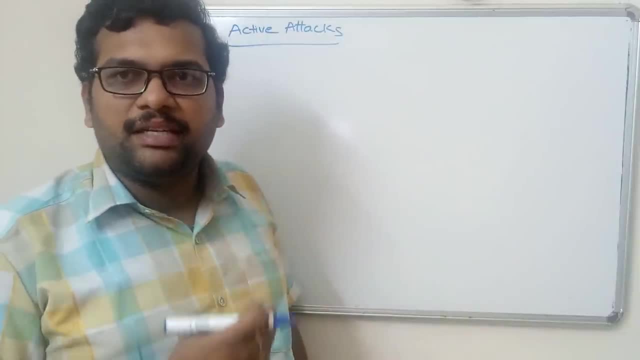 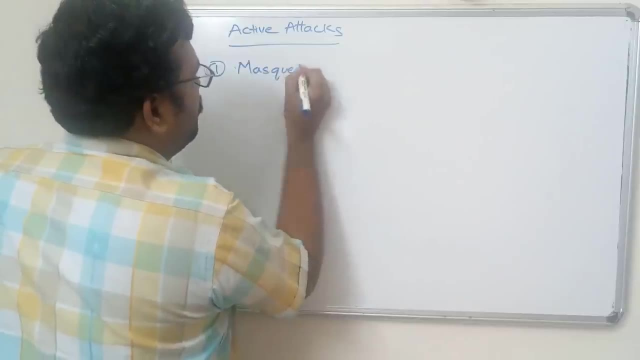 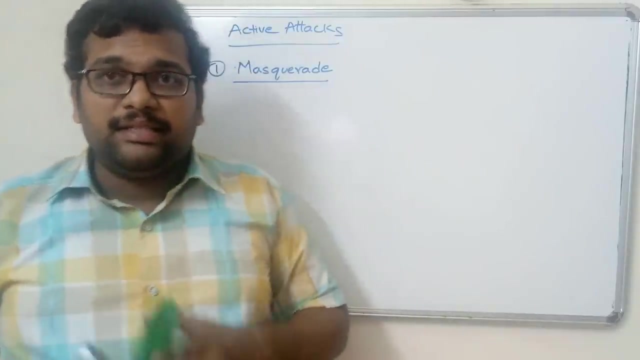 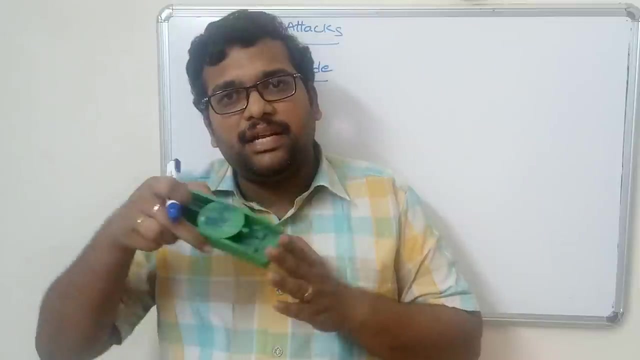 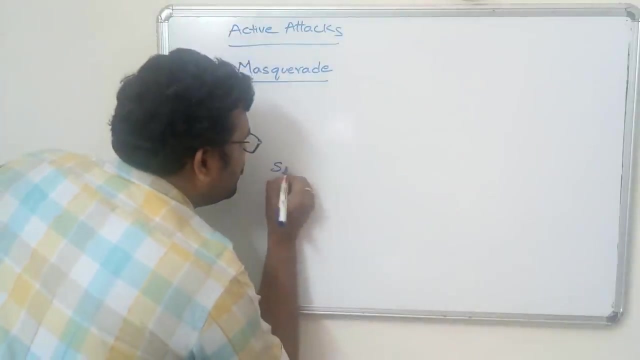 categories in this active attacks, four types of attacks. so first one is masquerade attack. masquerade attack. so in this masquerade attack the sender will sense the data to the receiver, so, but the receiver will receive the data from the third party on the name of sender. so this is the sender and this is the. 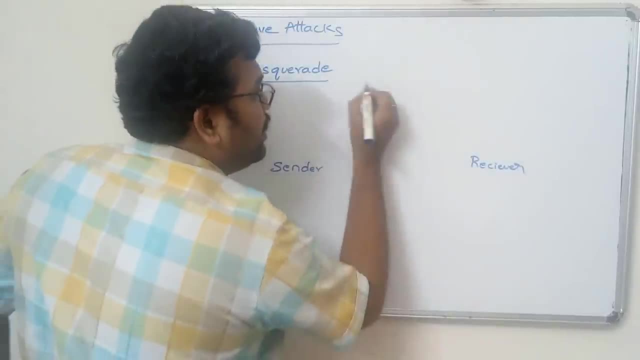 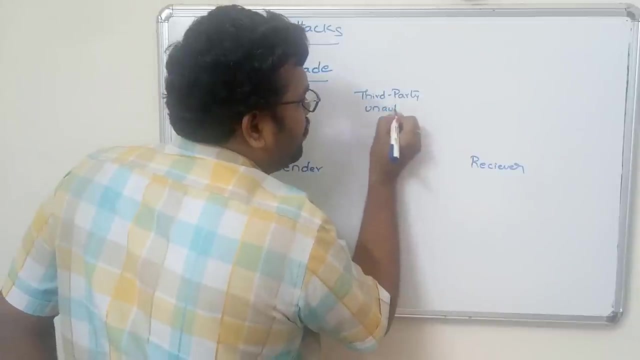 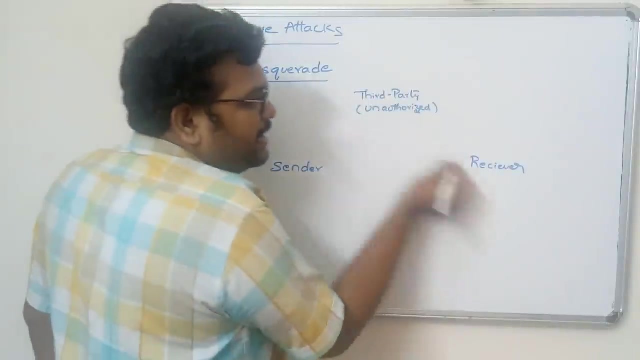 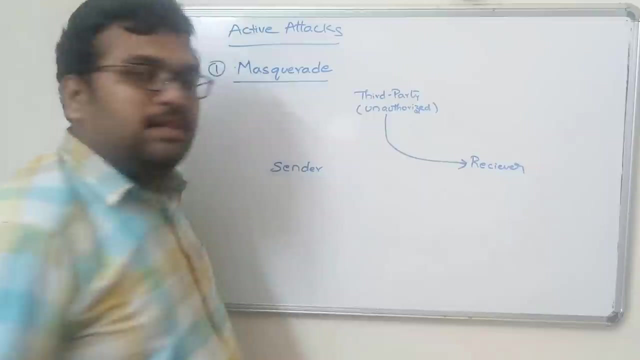 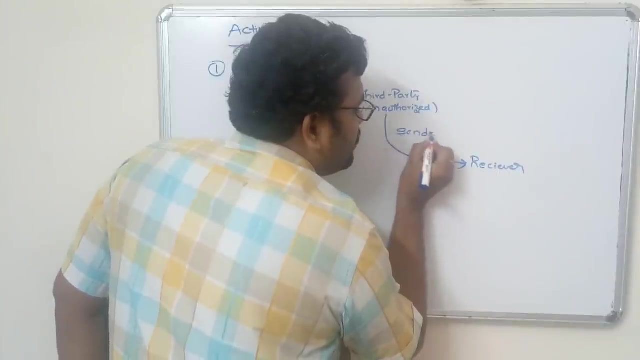 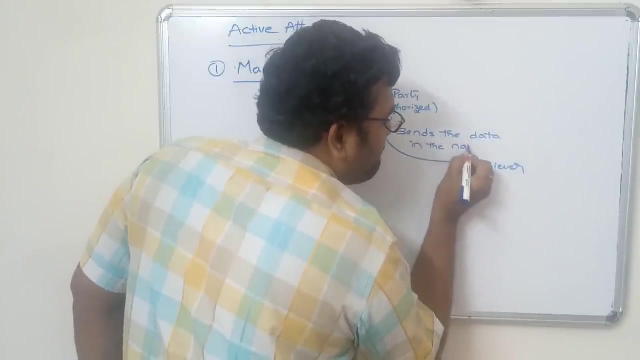 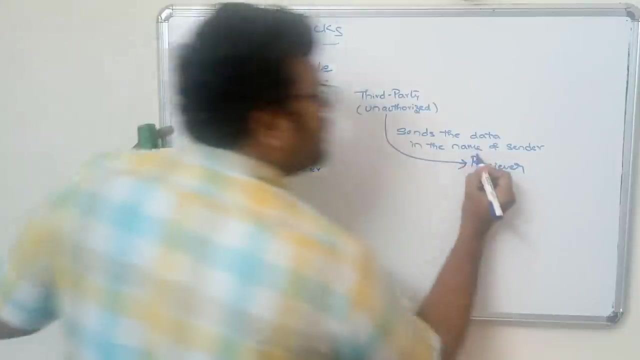 receiver and this is the third party. third party means unauthorized section, so this is the unauthorized person. so receiver will receive the message from the third party, from the third party with the name of sender, so sends the data in the name of sender. so the receiver don't know who will send the data, who is sending the. 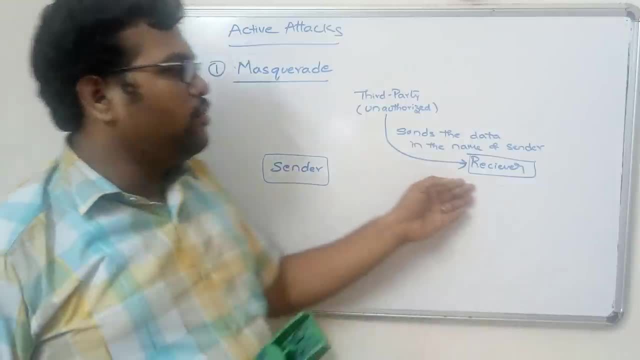 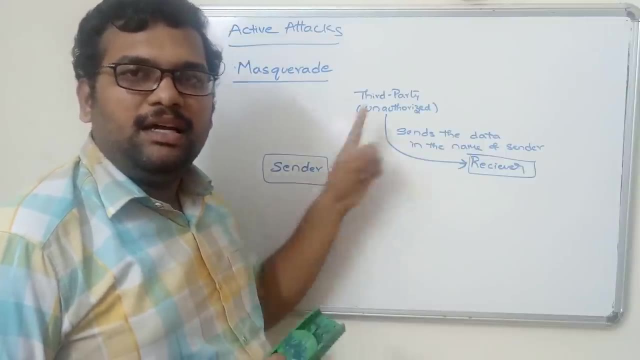 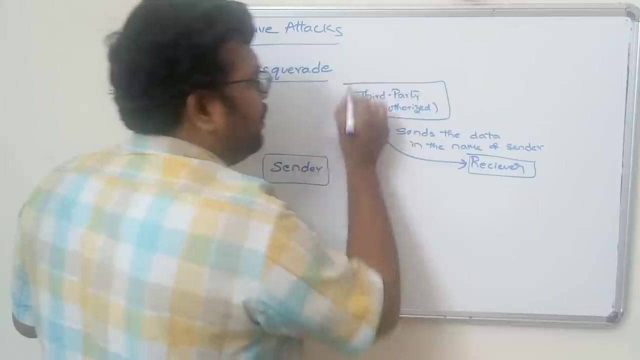 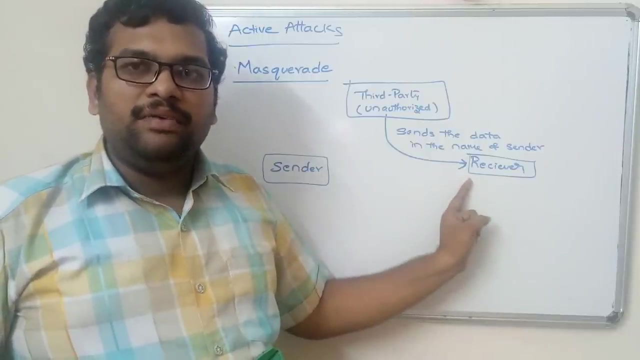 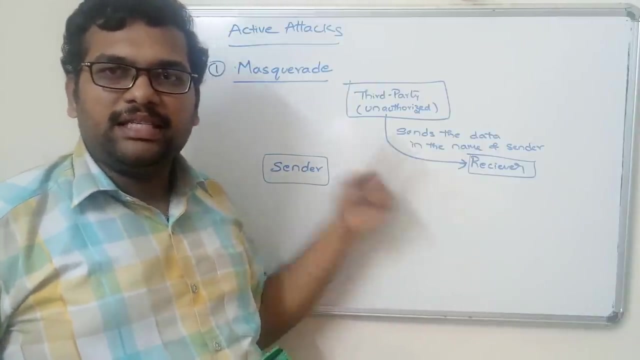 data. just the receiver will know that the data which was received was sent by the sender, but actually the data was sent by the third party. so the third party, that means unauthorized person, will send the data to the, the receiver, with the name of sender. so this type of attack, we call it as mask. 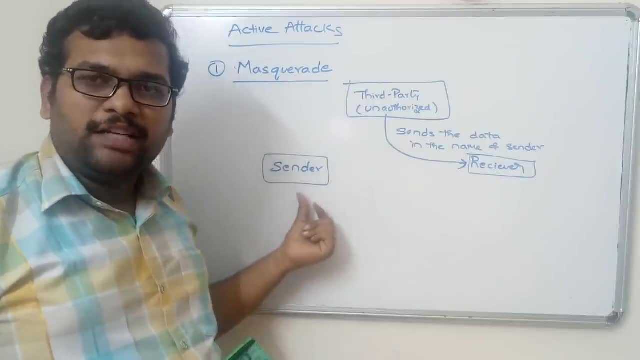 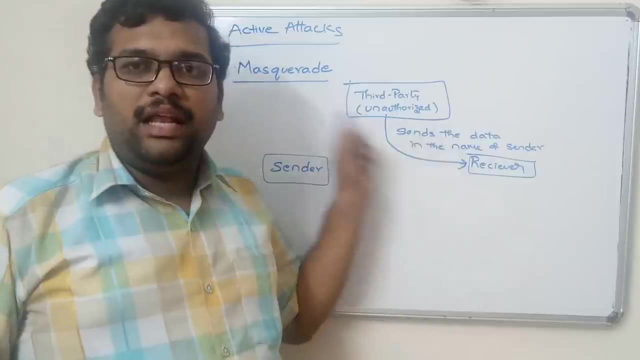 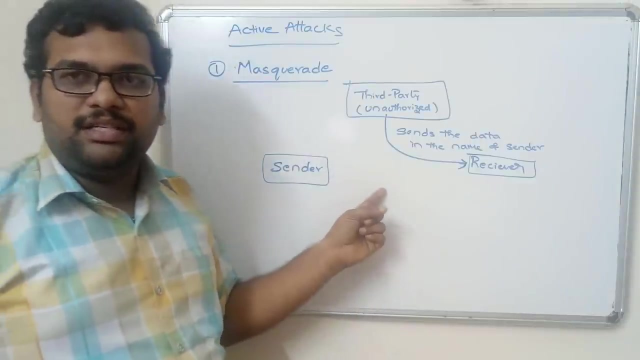 rate attack. so here the data is modified because actually the sender doesn't send that, there any data to the receiver, but the receiver was receiving the data with the name of a sender. so this type of attack we call it as a mask rate attack, and here the data modification is done. and the second one is: 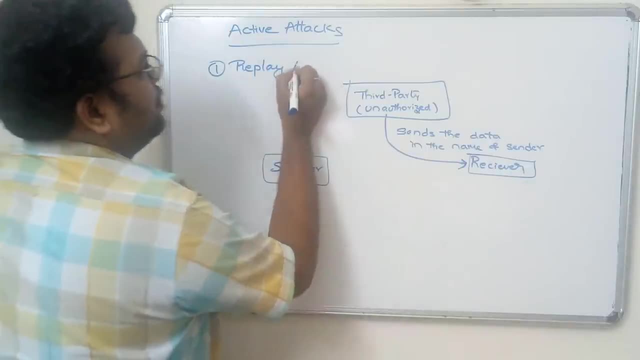 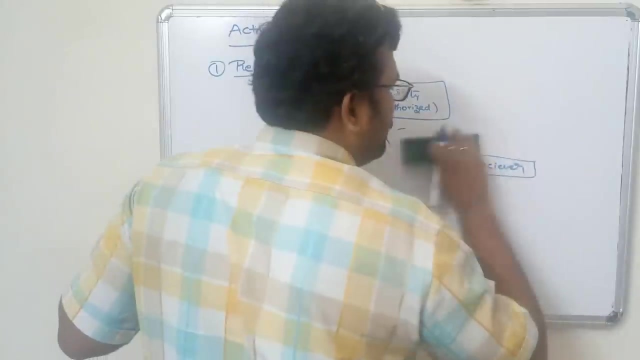 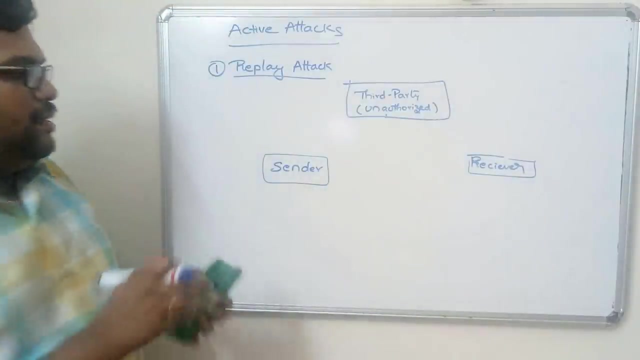 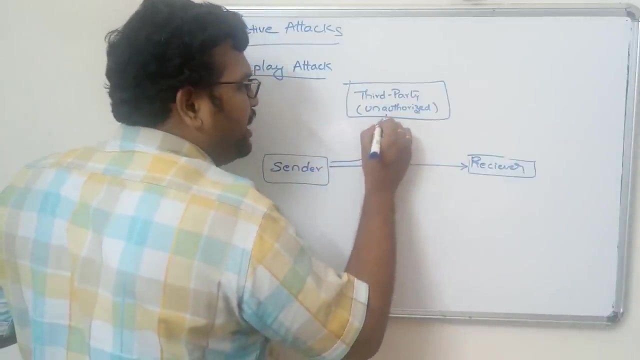 replay attack, replay attack. here again there is the sender and receiver, and again there is the sender and receiver, and and and and if. if the sender sends the message to the receiver and the same message will be gained by the unauthorized person and the modification will be done and the 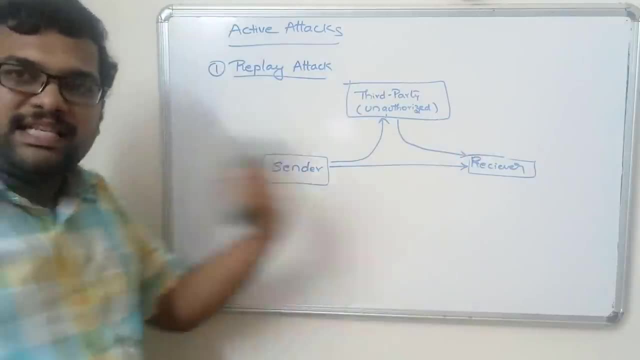 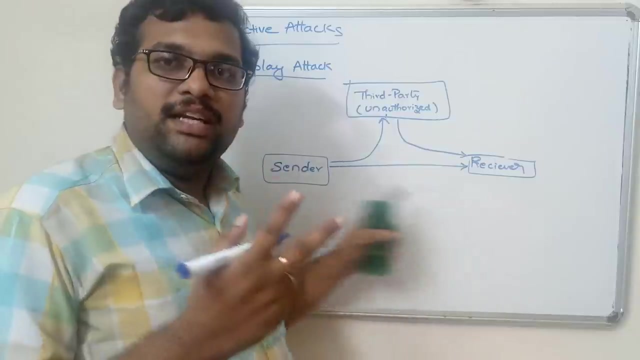 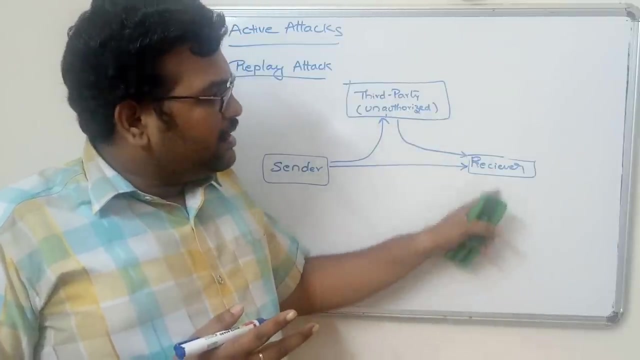 same message will be sent to the receiver once again. so that means a replay. so now the receiver will receive the message twice. one is from the receiver sender and one is from the unauthorized person. so receiver doesn't know which message is the correct message. that means, which message is the 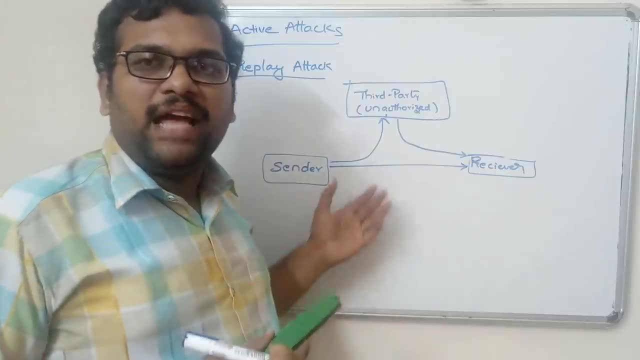 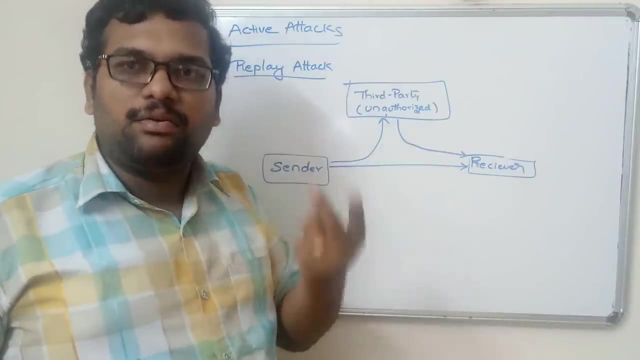 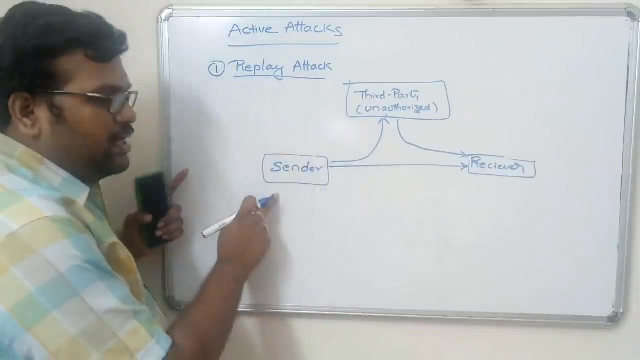 is the perfect message. that means which message was sent by the actual sender. because this receiver receives two messages, the same messages twice. so one is from sender, other one is from third party unauthorized. so sender sends the message to the receiver and the same message will be accessed by the 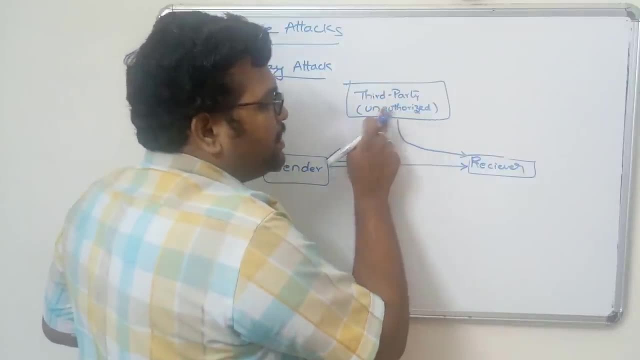 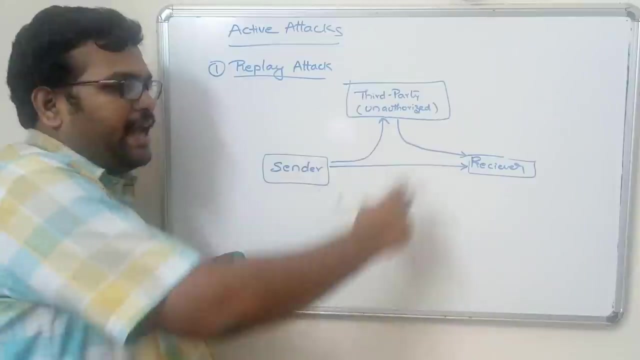 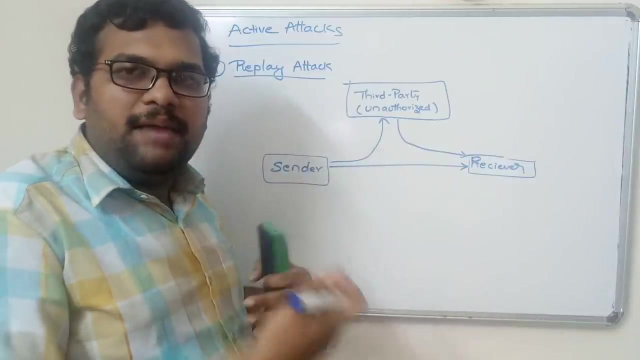 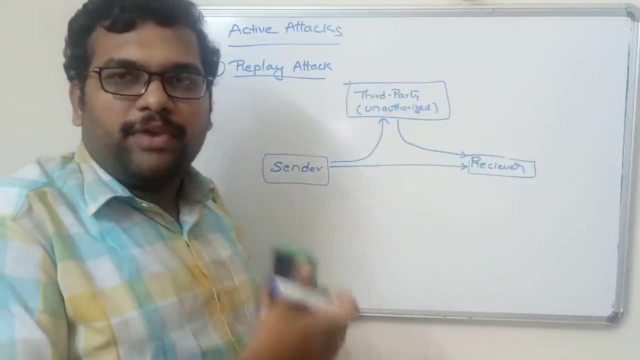 unauthorized person. and once again the unauthorized person will send the same message to the receiver. so this type of attack we call it as replay. the name itself indicates replay. so again and again we are sending the same message to the receiver. so that means the receiver receives the same message. number of. 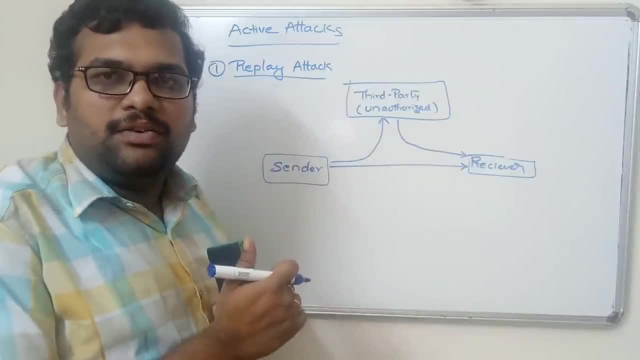 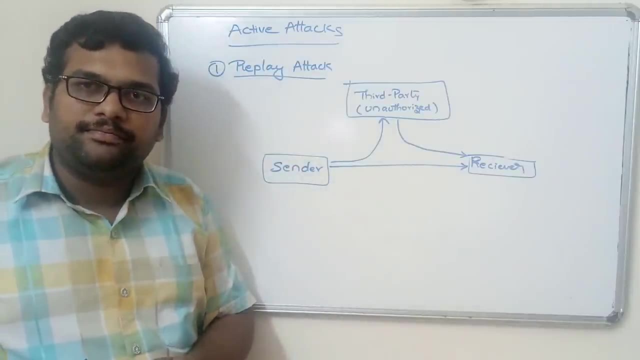 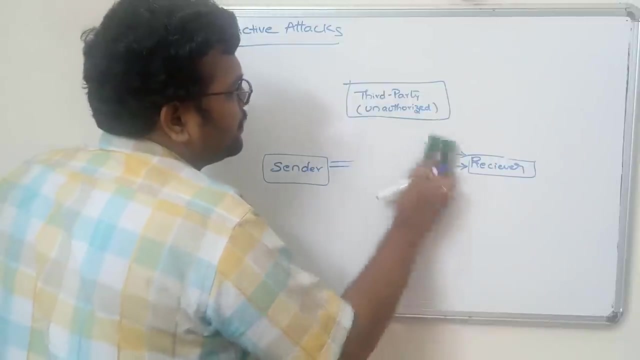 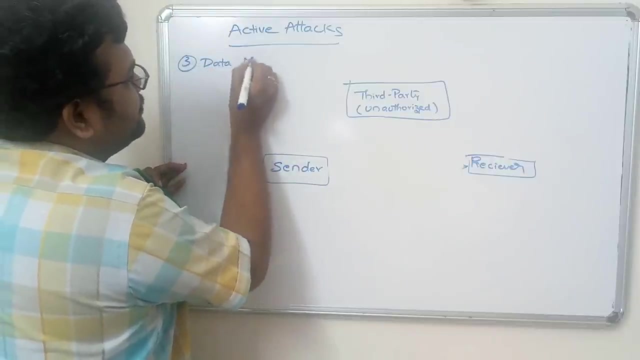 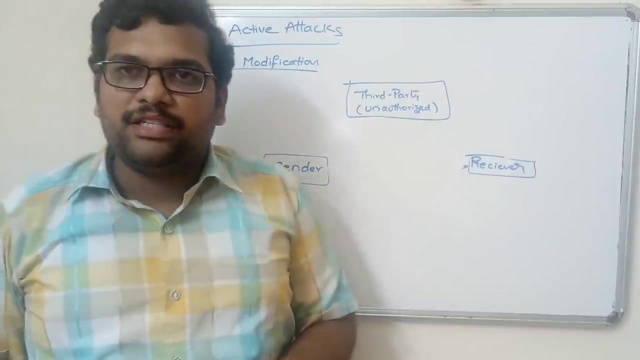 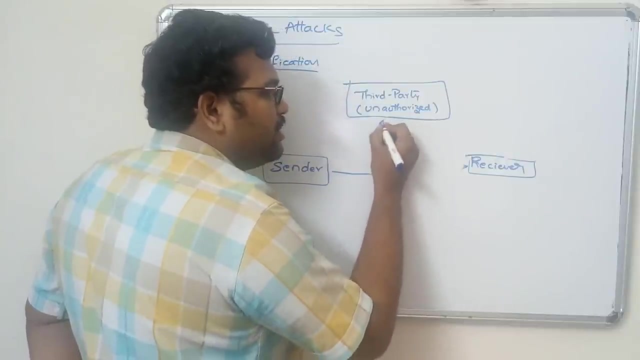 times and the receiver doesn't know which one is the correct message. so this is here also, the modification is done. and the third one coming to the third one: data modification. data modification- here also, the sender sends the data but it doesn't go to the receiver. that message will directly accessed by the third party and 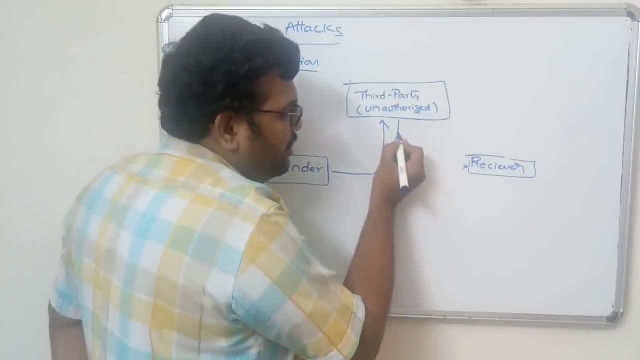 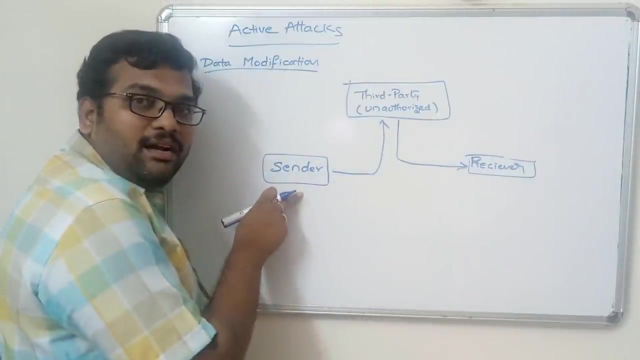 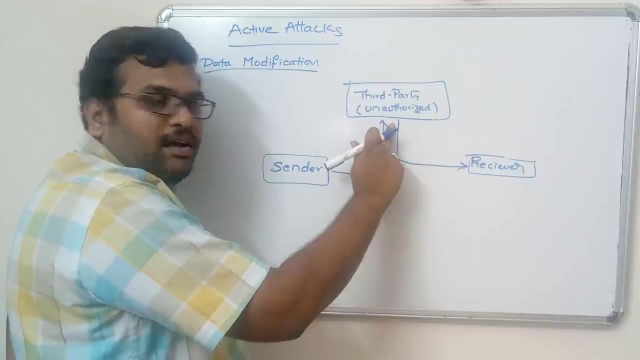 modification will be done on that particular message and again, this message will be sent to the receiver. so the data which was sent by the sender will be received by the unauthorized person and the data will be modified and the modified data will be sent from the unauthorized person to the receiver. so 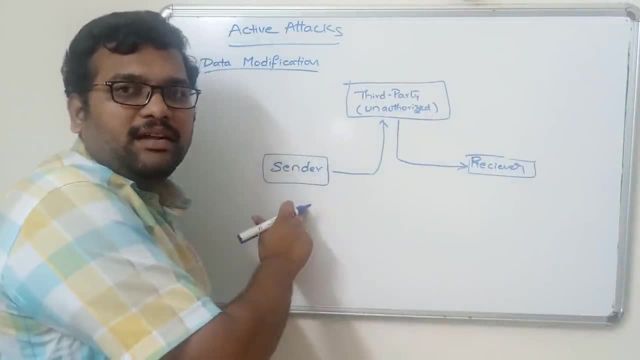 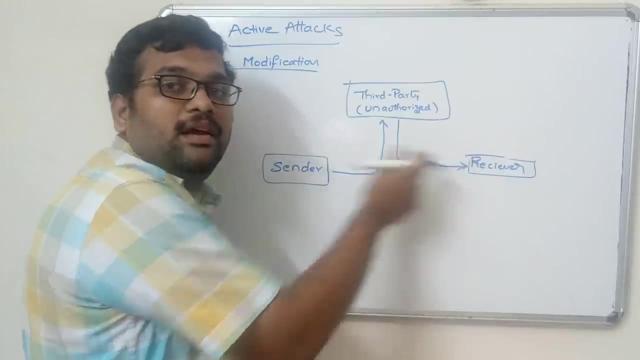 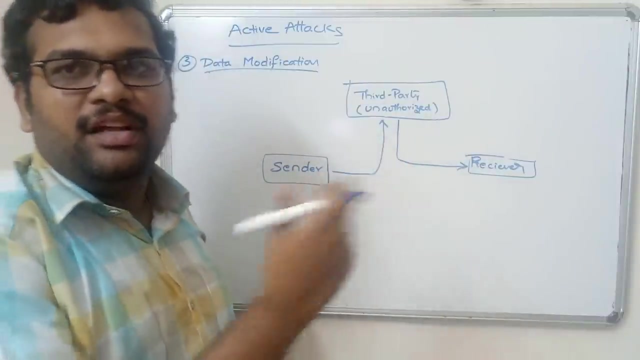 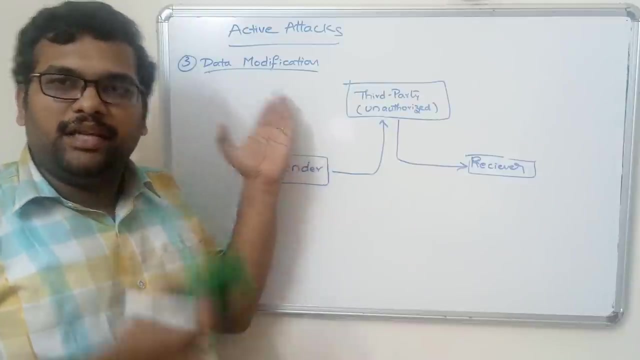 all these messages will be within the name of sender. so whatever the message this unauthorized person sends to the receiver will be in the name of sender. so receiver doesn't know. there is a modification on data during the transmission, so that's why we call it as an attack. so data modification, attack. so here name. 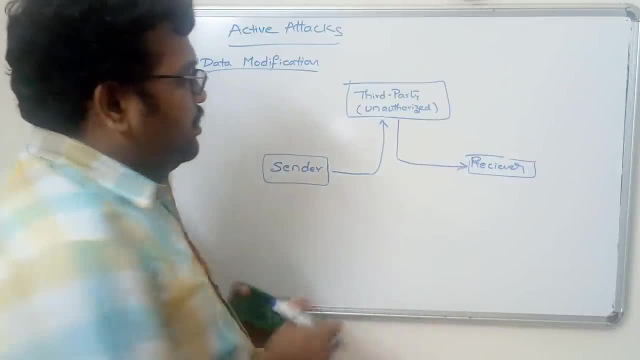 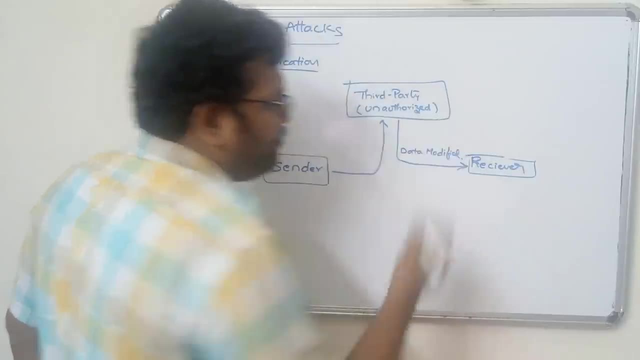 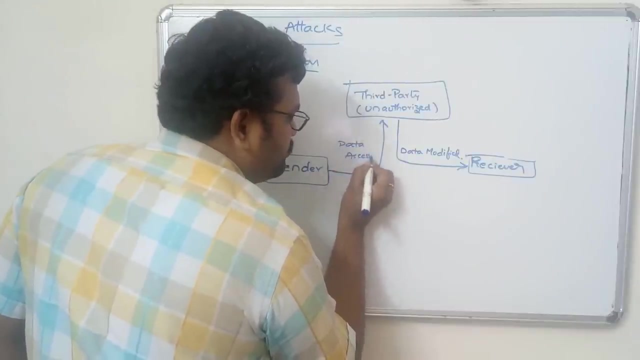 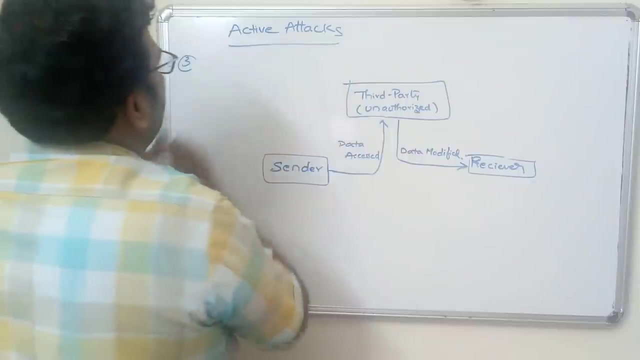 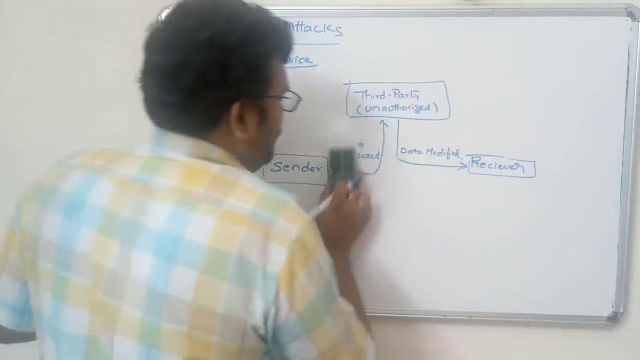 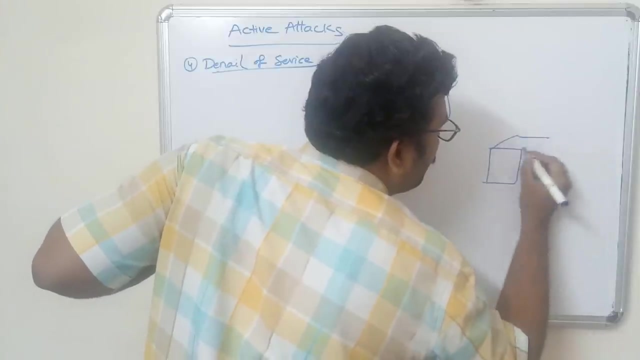 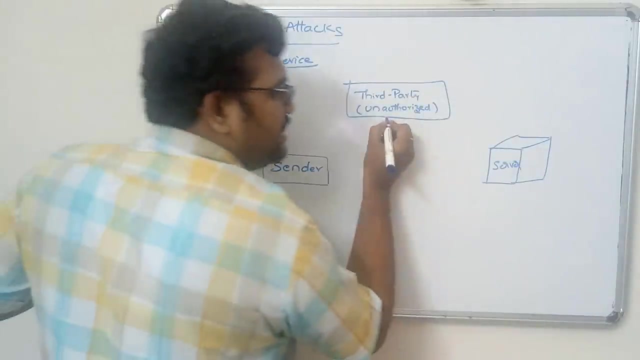 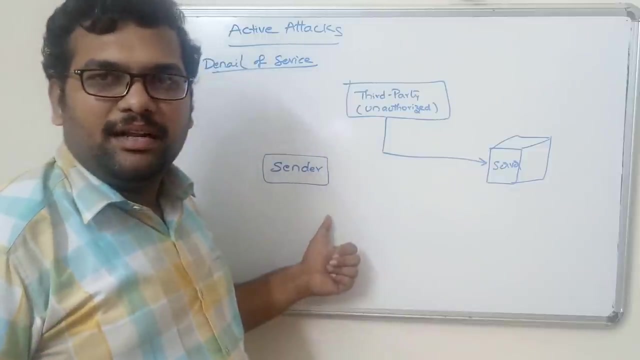 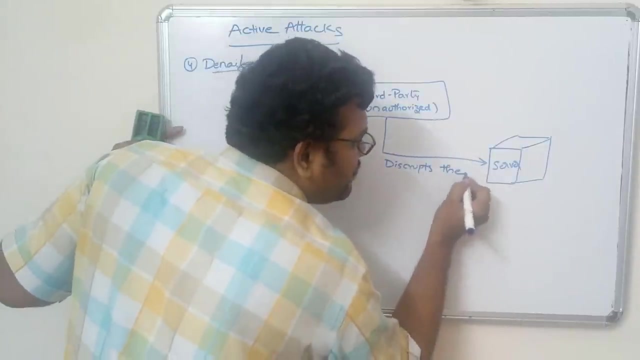 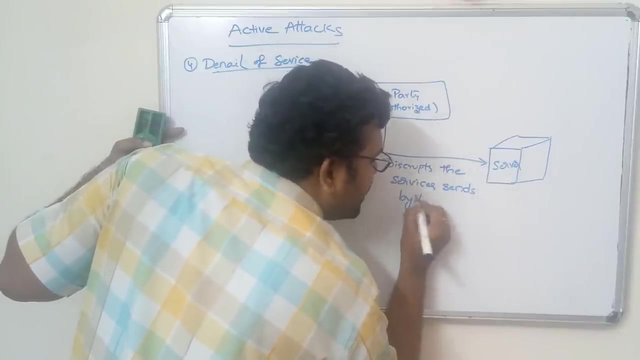 itself indicates there is a data modification. so here the data is modified and here the data is accessed right. and the last one is delay of service, denial of services here. So this third party will interrupt the services which are sent by the server to the sender. So it disrupts or interrupts the services sent by the server.